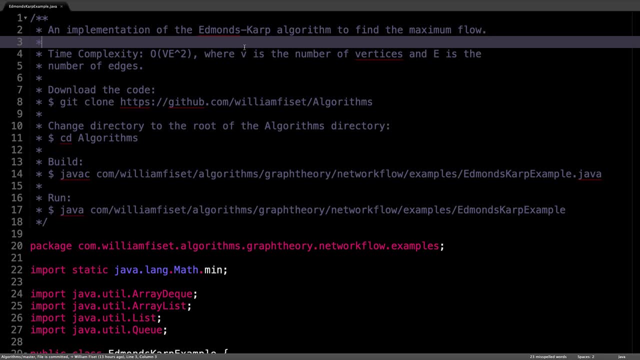 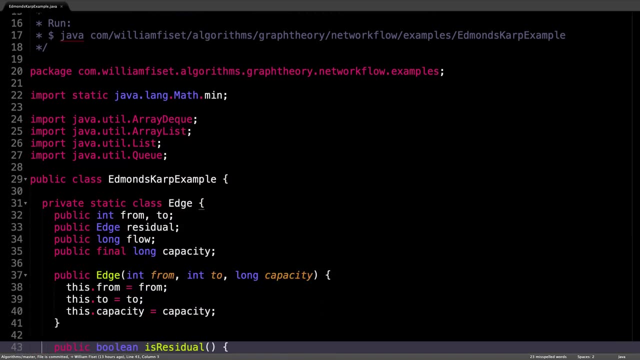 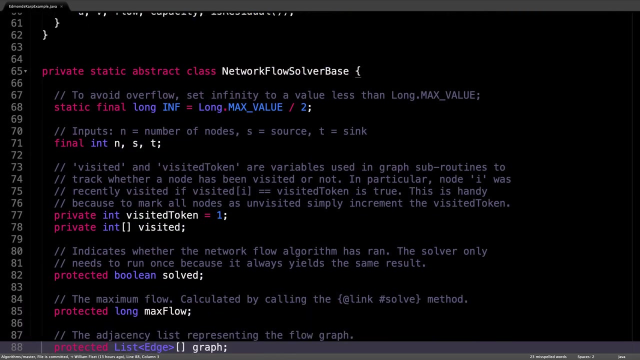 laid out some instructions here in the header in case you wanted to download the code, play around with it and run it yourself. If I scroll down, you can see that we still have the same setup as before with the edge class Right here and the network flow base solver. But there is one important change I have made. 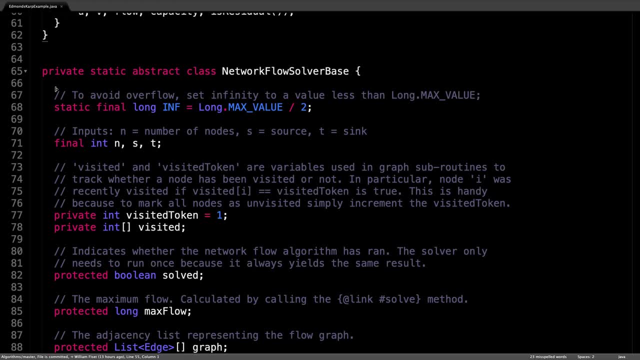 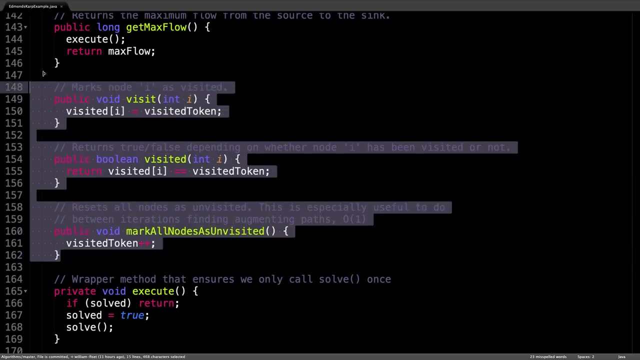 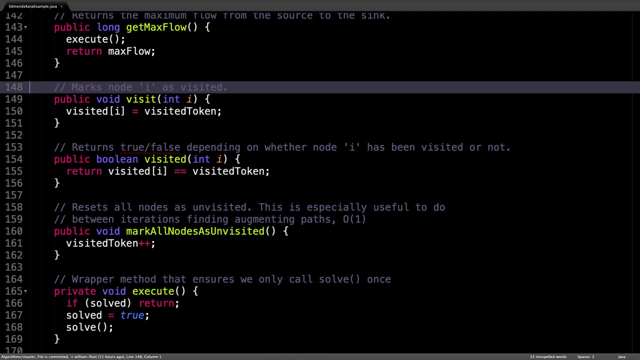 since the Ford Fulkerson video, And that is, I have added three new methods. If we scroll down, you can see that the three new methods are right here, The three methods I added: abstract away, visiting nodes and marking all nodes as unvisited. Now this is all done efficiently. 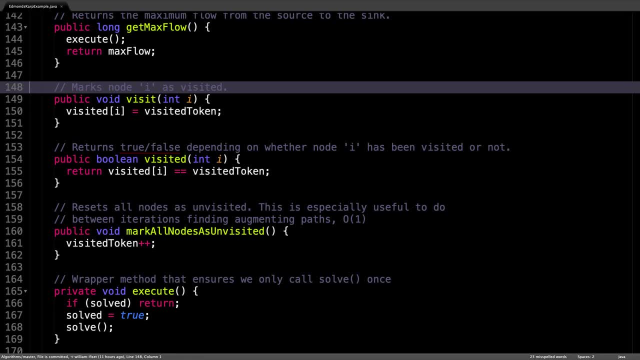 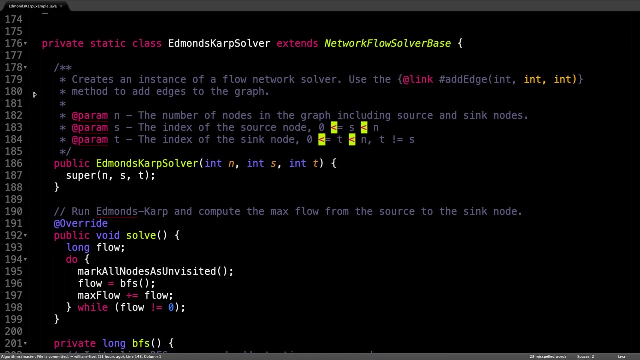 internally through the network flow base solver class using a visited token. you don't have to worry about It. also helps readability for anybody who's new to the code. Alright, now let's have a look at the Edmonds carp solver, which is the only thing different in this file. 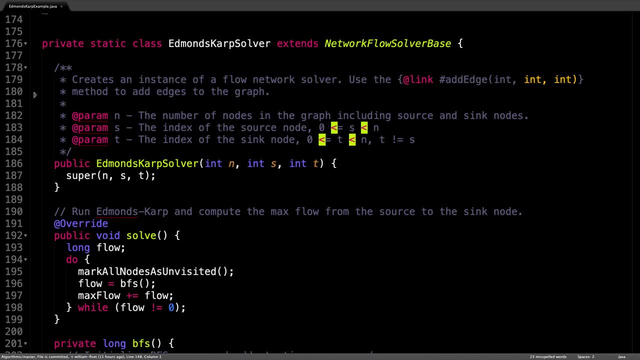 First notice that the Edmonds carp solver extends the network flow solver base. In doing so, we get a whole bunch of things for free, including the ability to construct a flow graph before we push flow through it. In the constructor for the Edmonds carp solver, all I do is call the superclasses constructor. 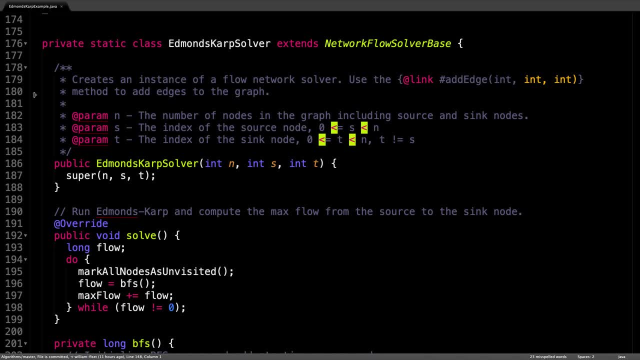 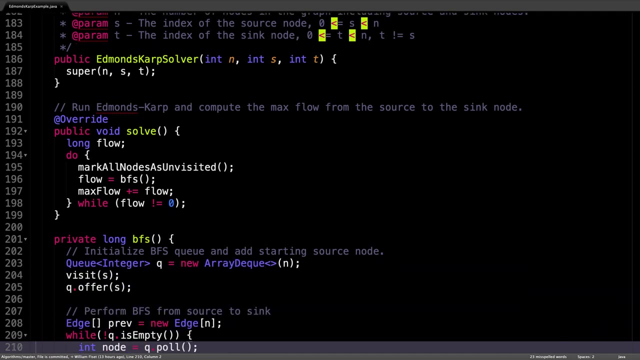 This performs various initializations, including allocating memory for the flow graph and registering which nodes are the source and the sink. The most important method in the Edmonds carp solver is the solve method. right here The solve method is called just before we get the maximum flow. This method is really short. 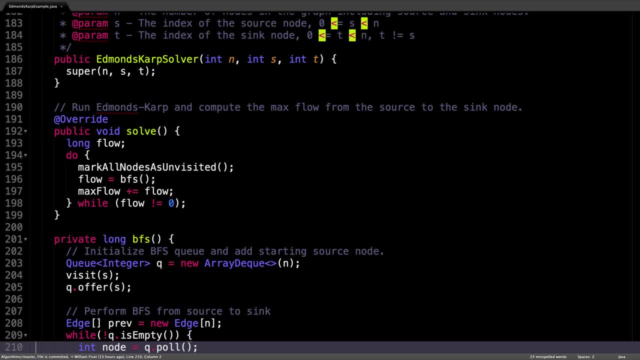 All we do is repeatedly find augmenting paths from the source of the sink until the flow we get is zero, at which point we know that the graph is fully saturated and no more augmenting paths can be found Line by line. what we do is mark all nodes as unvisited before each. 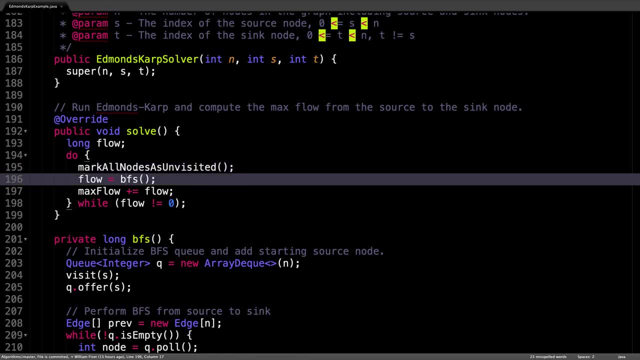 iteration, run a breadth: first, search and get the bottleneck value and then some overall bottleneck values to calculate the maximum flow. Now let's take a closer look at the flow. Now, let's take a closer look at the flow. In this example we have a graph that is: 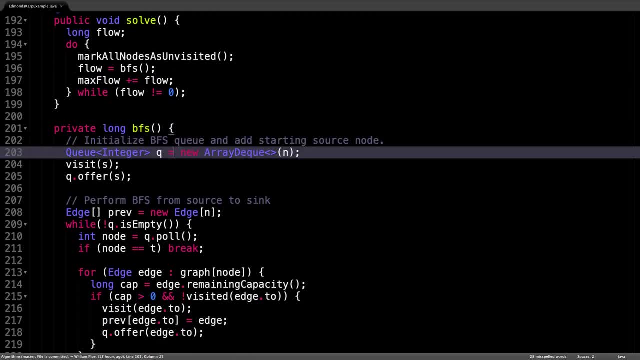 one of the most important nodes in the queue. So let's take a closer look at the breadth first search method. The first thing I do is initialize an empty queue data structure, because I know that we're going to need one to do a breadth first search After the creation. 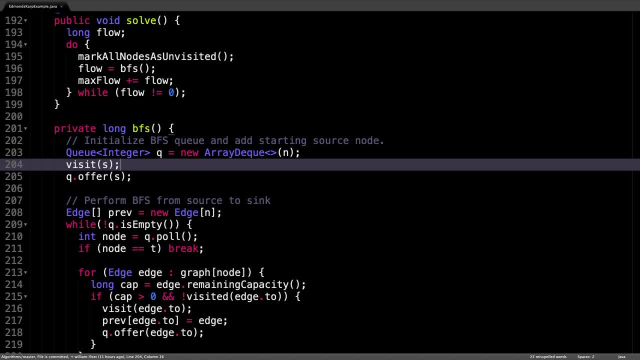 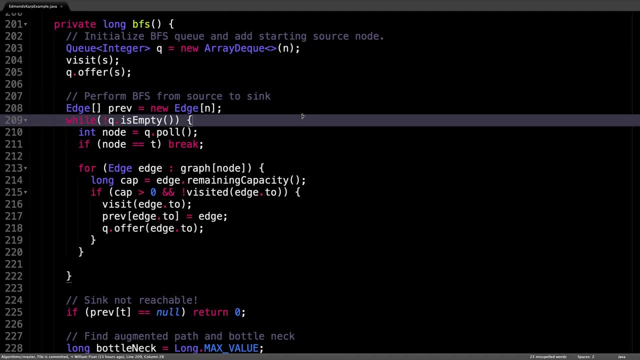 of the queue. what I do is I visit the source node and add it to the queue so that the breadth first search starts at the source. Then do your standard breadth first search loop. while there are still nodes in the queue, remove the first node found in the queue If it's. 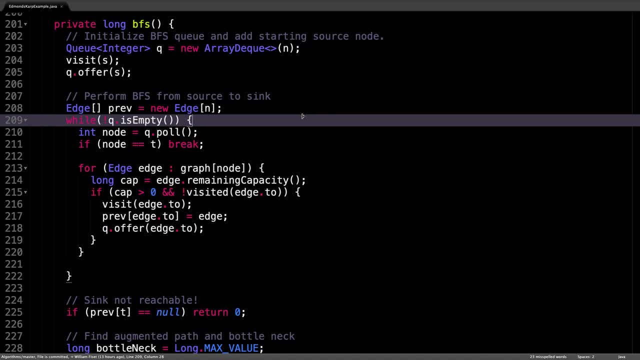 the sink stop, otherwise iterate through all valid adjacent neighbors. we can add a node to the queue If it is not already visited and the edge leading to the node has a capacity greater than zero. However, before we add the node to the queue, we've visited and track. 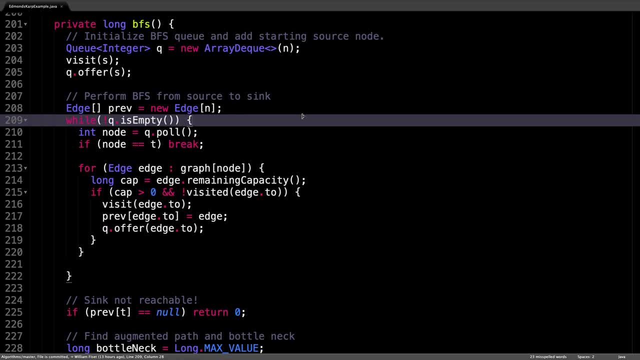 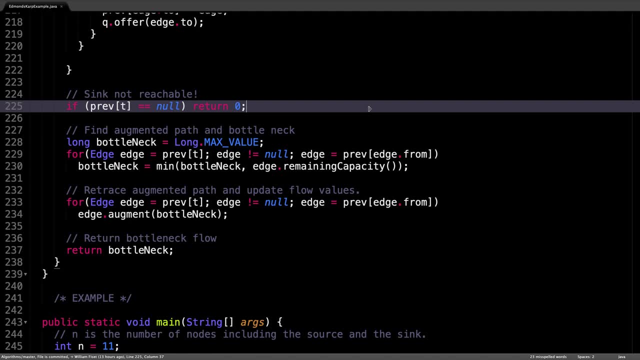 where it came from by placing an edge in the prev array to rebuild augmenting path later on. Alright, so moving on. We know that the breadth first search did not actually make it to the sink. if we have no entry at the index of the sink in? 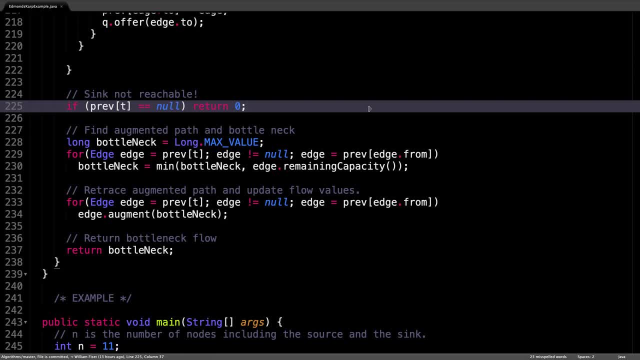 the prep array So we can return early after this point. we know that there exists an augmenting path. Since we know an augmenting path exists, we can find the bottleneck value, that is, the smallest remaining edge capacity along the path. We do that by starting at the sink and 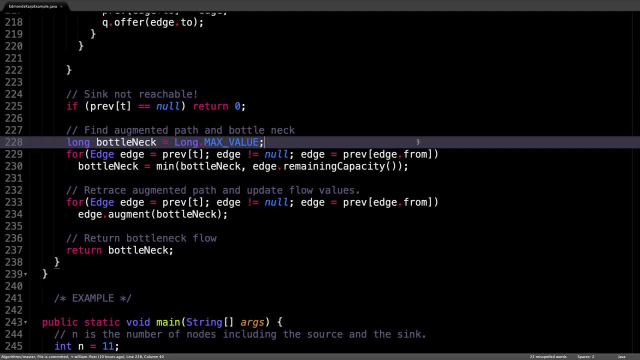 reconstructing the augmenting path, going backwards by repeatedly reaching into the prep array until we are back at the source. then we need to update the flow along the augmenting path to adjust the flow values, So once again loop through the edges forming the augmenting 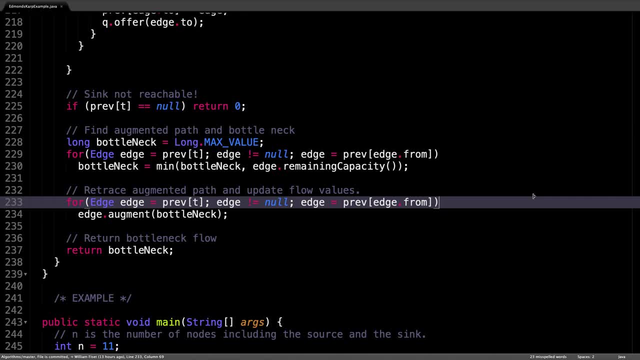 path. then the augment method takes care of increasing the flow along the forward edges and decreasing the flow along the residual edges. The very last thing to do is to return the bottleneck value so that we can sum the max flow and the solve method, And that's. 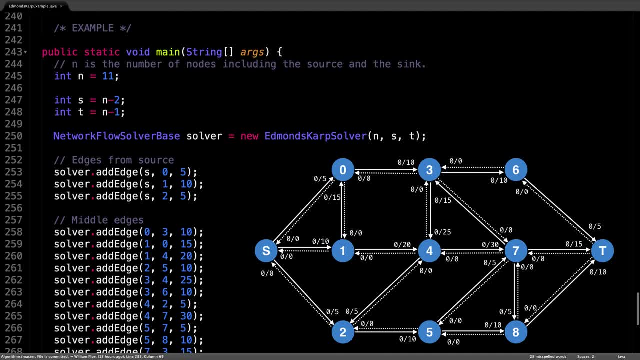 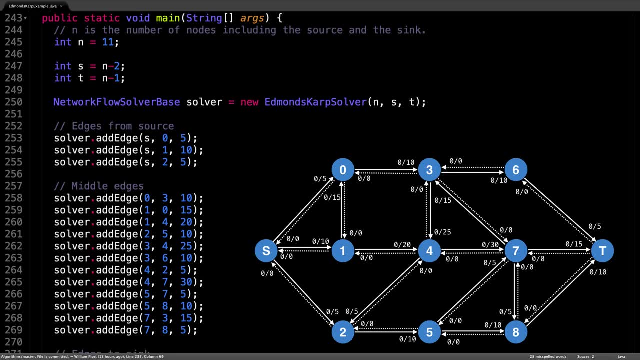 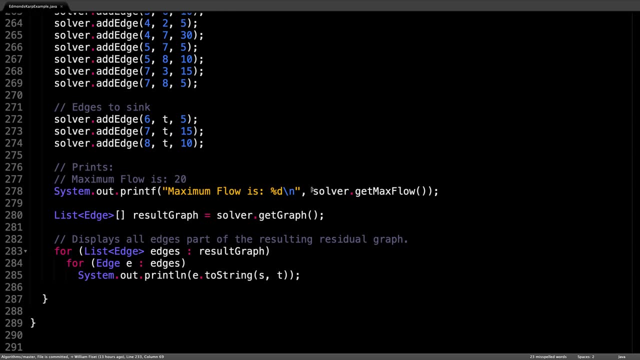 basically it for admins cart To actually build a flow graph. have a look at the example right here in the main class. It sets up the flow graph from the previous video and pushes flow through it. You can see down here where we actually create the solver and run the solver to get the maximum. 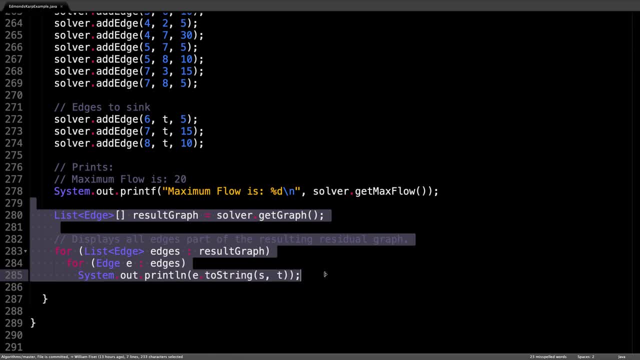 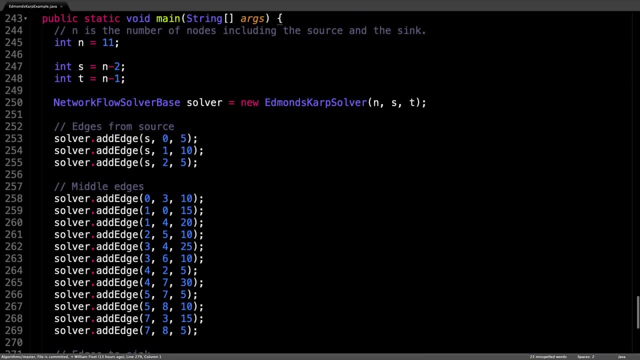 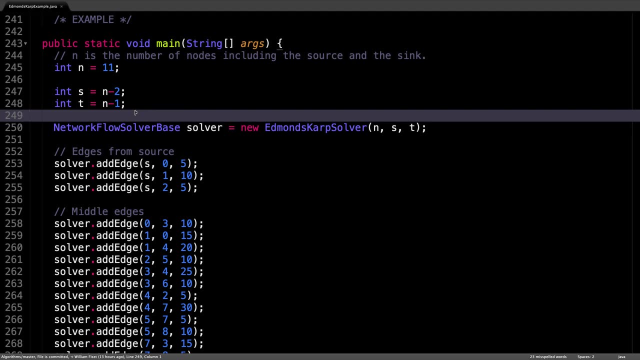 flow and then finally display the resulting graph after the maximum flow has been pushed through it. So this is really handy to understand. So please have a look at this in more detail if you're struggling to understand Edmonds carp- Awesome. Thank you for watching. Please like this video if